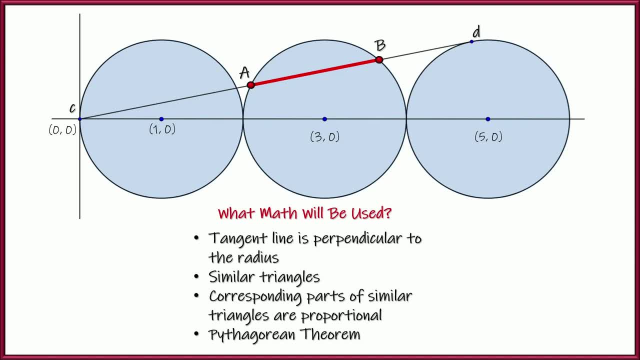 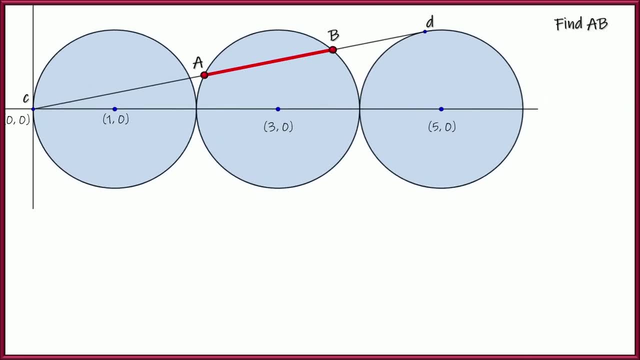 and you'd like to try it again. with these clues in your back pocket, go ahead and dive in, because in about three seconds, two and one and dive in. All right, we're looking for the distance of a to b. A good idea, a good way to start, is to see if you can express. 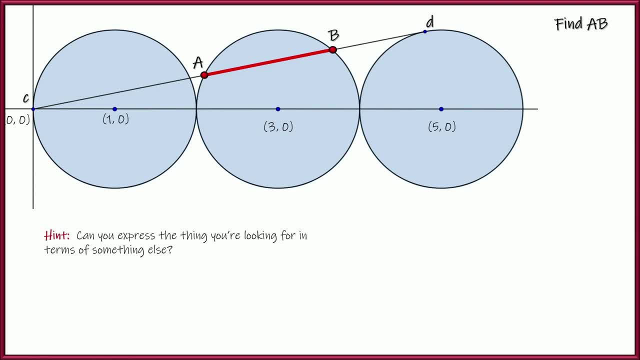 the thing you're looking for in terms of something else. Now, when I did this problem, I wasn't really sure how to even start, so I just started by saying, hey, let's make this an isosceles triangle, because if I have an isosceles triangle, I can drop a perpendicular bisector like this. I know it's. 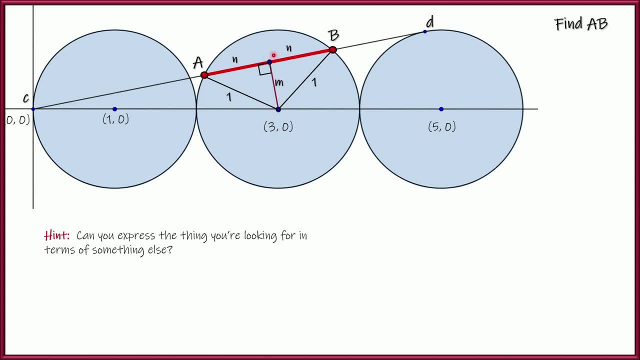 isosceles, because if I have a perpendicular bisector, I can drop a perpendicular bisector because it's the radius either way. So here's what I've got. now I know that this side n is half of a- b, so a b is 2n. All right. now the other thing is, these problems rarely give you information that. 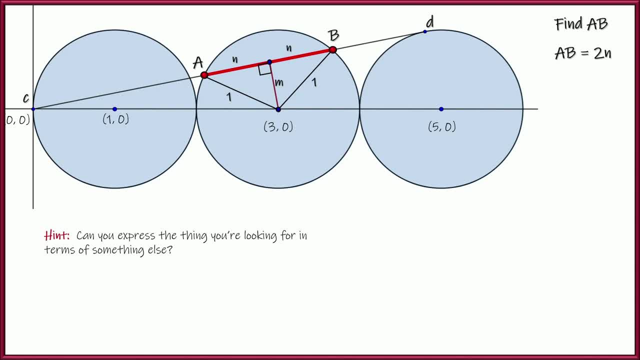 you don't have to use. So cd is tangent to the circle over there with the radius of one, with the center at five zero. So if I draw that radius I know it's perpendicular, because tangent lines are perpendicular to the radius at the point of tangency. That means that these two line segments 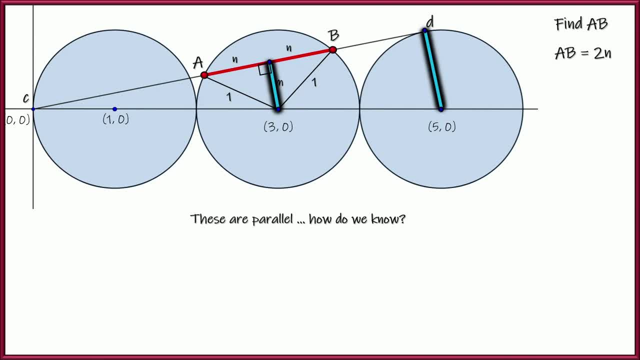 right here. these two are parallel to each other and the reason I know that is they're both perpendicular to the same exact line. And I know they're perpendicular because, once again, cd is tangent, so tangent is perpendicular to the radius at the point of tangency. All right, that's pretty. 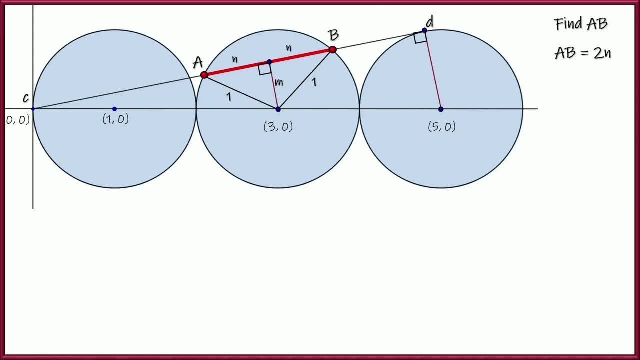 cool. So we got a right angle there. we got a right angle there, and the reason that that's important is because it's going to be perpendicular to the same exact line. So if I draw that line, it's going to give us a pair of similar triangles. Do you see this little angle over here? We've got. 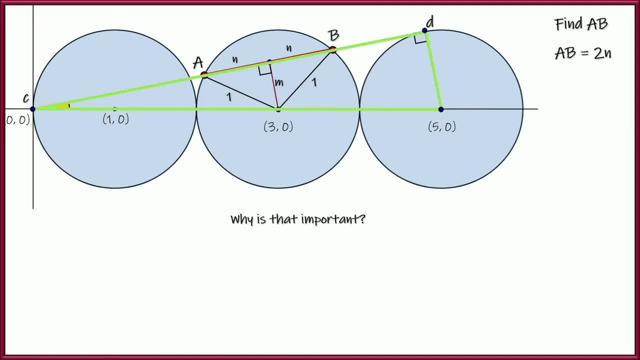 two triangles here that are similar. they both have right angles and they both share that angle. So all three angles are going to be congruent, which makes the triangle similar. So let's go ahead and explore those two triangles to make sure you really see it. There's the first one right there. 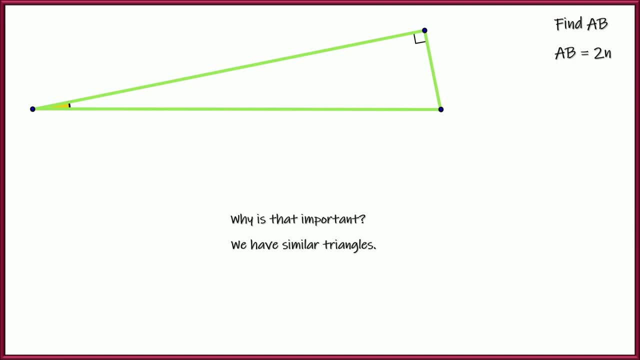 it's the biggest. one goes to the center of the circle, that is, at five comma zero, and the other one's at three comma zero. So these two overlap. That's how they look If I separate them, just in case you don't see it. that's exactly how they are. 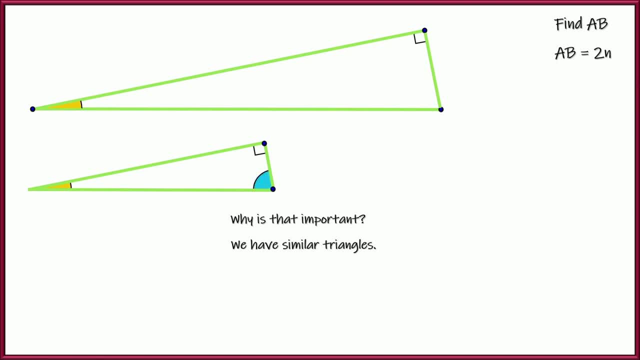 And I know that they are similar because all three angles are going to be the same. If I know that they're both right angles and these two are the same angle because they overlap, then the other angles have to be the same. So let's go ahead and put it back on top of our original diagram so that 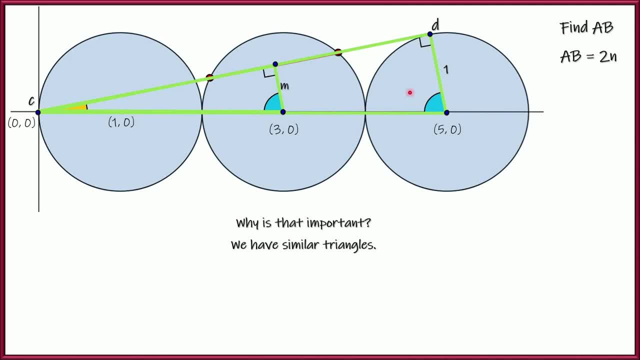 you can see what I'm talking about, how it fits together. All right, so we have two similar triangles. That means the corresponding parts of similar triangles are proportional. So I know M is equal to 1- 5th. Now let's see where those numbers come from. The five over here is that. 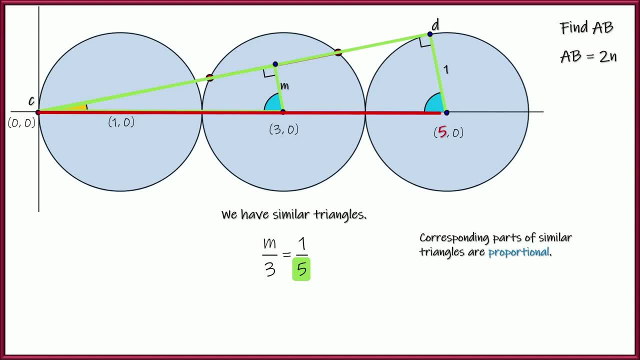 bottom side is the hypotenuse of the biggest triangle and the three is the hypotenuse of the smaller triangle. So those are corresponding parts and the M and the one. well, those are the side legs over there, those kind of ones on the right hand side for us, M and one. So this is our. 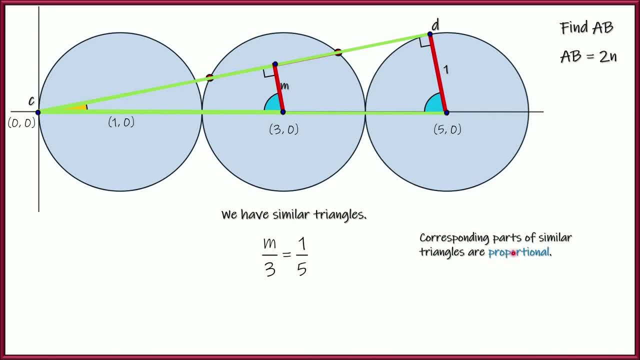 proportion. right here. Proportions are equal ratios, Ratios are fractions. So when you see things are proportional, what you're saying is you have two fractions that are equal. You can solve that real easy. Multiply both sides by 3.. M is equal to 3 5ths. Tuck that away over. 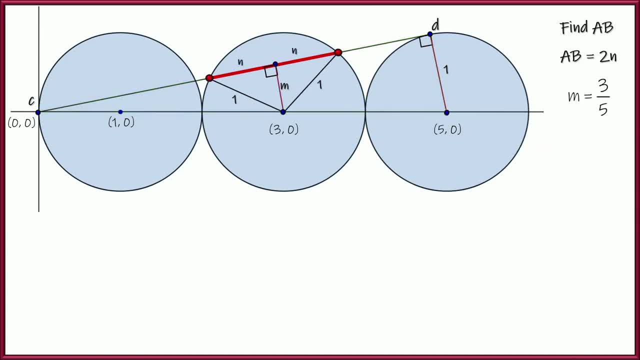 here and kind of reconstruct our original triangle there. All right, so we know M is 3, 5ths. So what we're going to do is we're going to use the Pythagorean theorem. Let's go ahead and just look at one of those triangles and solve for N and then double it, right So Pythagorean theorem. 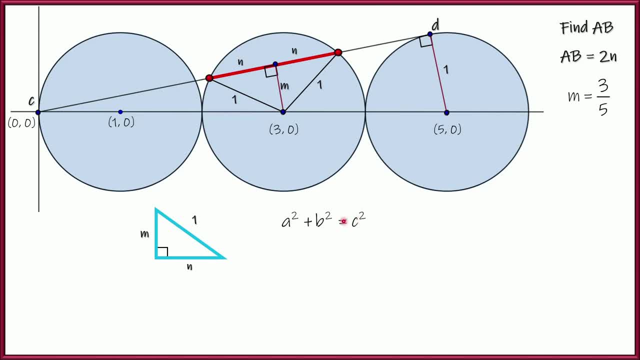 A squared plus B squared is C squared, of course, right. So the hypotenuse is 1. The legs are M and N, So we're just going to plug those in And solve for N. I think it's always a good idea to solve for the thing you're looking for. 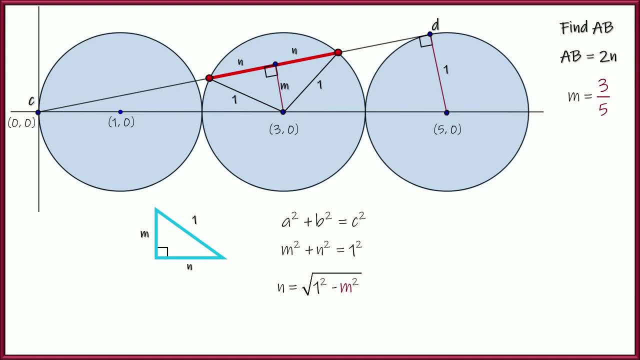 before you plug in the values Makes things just a little cleaner. So now we know M is 3- 5ths, So we're going to plug in 3- 5ths. Let's go ahead and square all that: 1 squared is 1.. 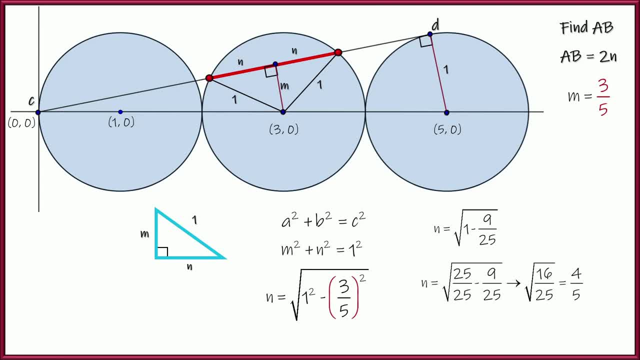 3- 5ths squared is 9- 20- 5ths. You got to get a common denominator right: 25 over 25 minus 9 over 25 is 16 over 25.. And the square root of 16 and 25 is 4 and 5.. So N is equal to 4 5ths. 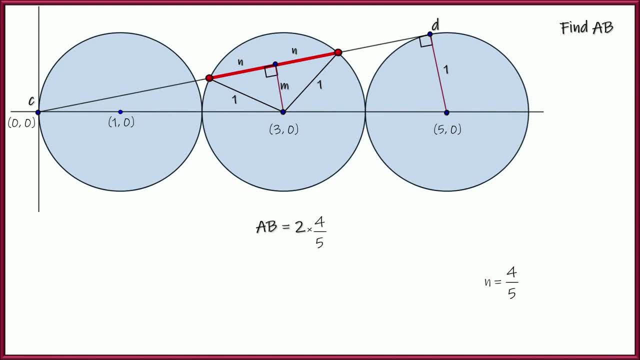 Double. that Double of 4 5ths is of course 8- 5ths. So our answer A to B That's 8 5ths. That's pretty cool, right, Hey? if you like this video, do me a kind favor, Like subscribe.